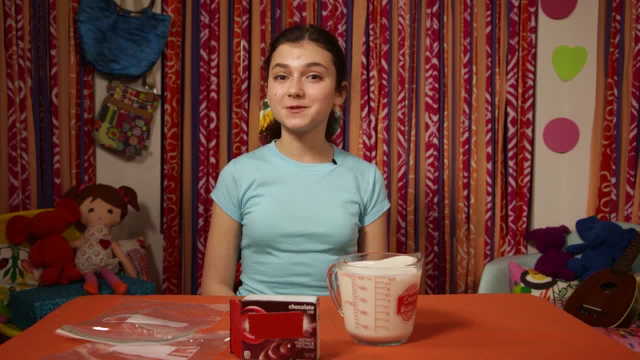 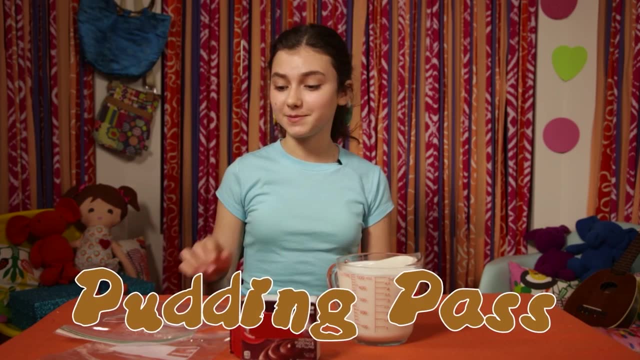 The outdoor fun has just begun. This next hack makes fun in the sun a real treat Time to play with our food. with this hack I call Pudding Pass. For this you'll need some ziploc bags, instant pudding mix and some milk. 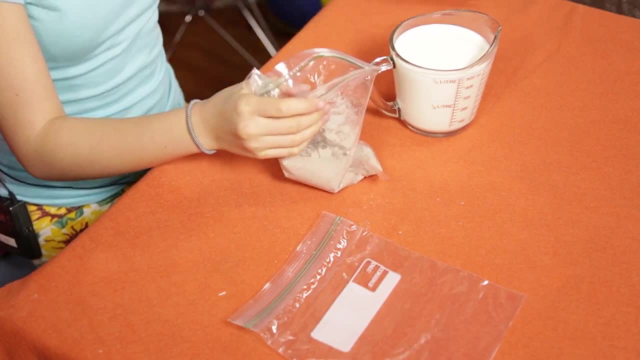 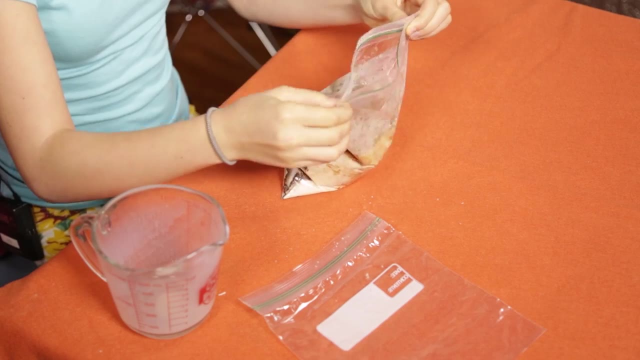 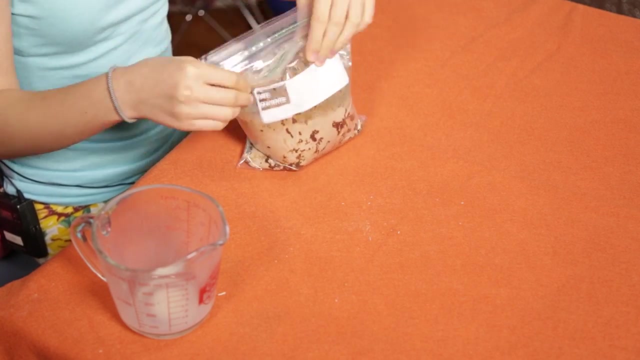 Combine the dry pudding mix with milk, just like it says on the pudding box. Only this time you pour the ingredients into a plastic bag instead of a bowl. Now double bag it for safety. Then head outside and play Pudding Pass with the bag until your pudding is ready to eat. 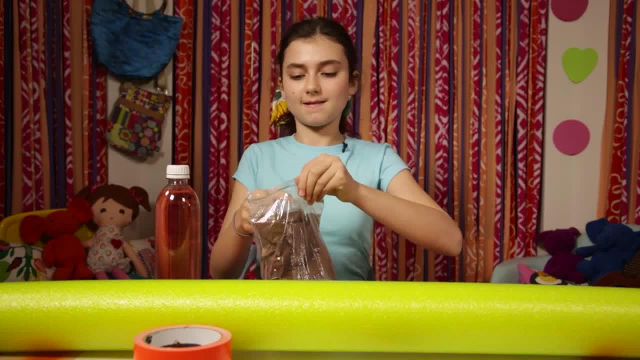 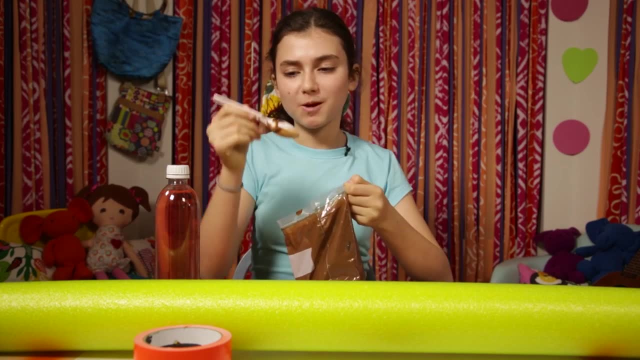 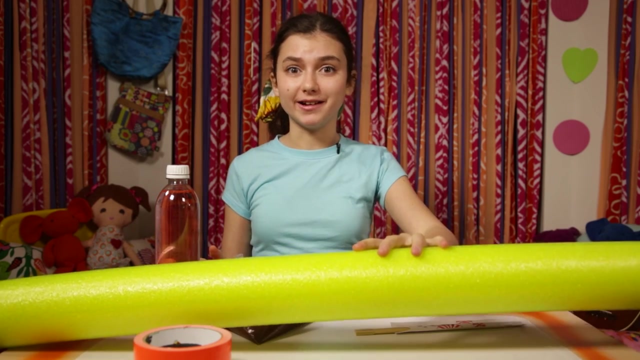 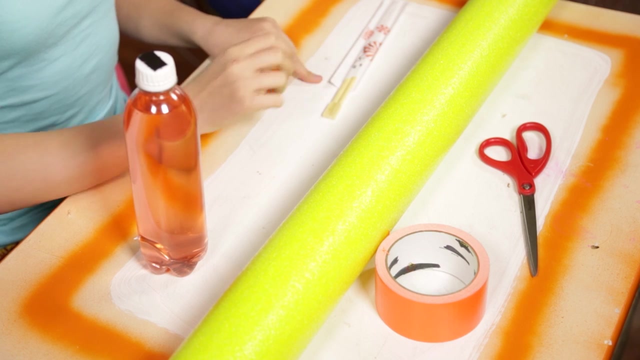 Ready to eat. In the video below, I showed you how to make your favourite pudding Yummy. For my last hack, I'm using my noodle, Literally. Let me show you how to make my noodle sprinkler. For this you'll need a bottle cap, chopsticks, a pool noodle, duct tape, scissors and a hose. 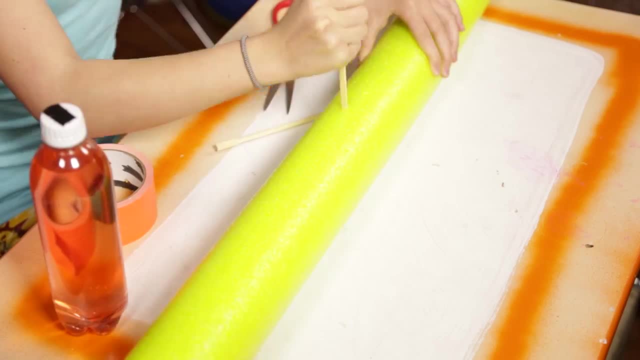 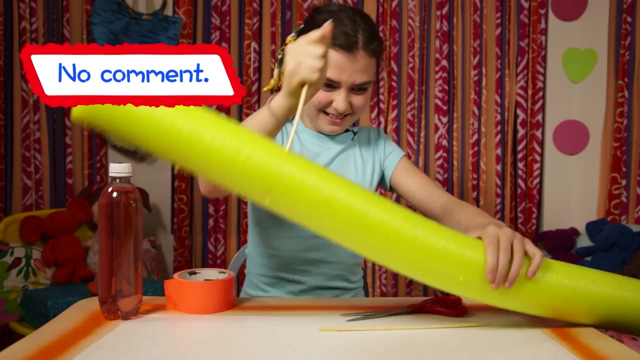 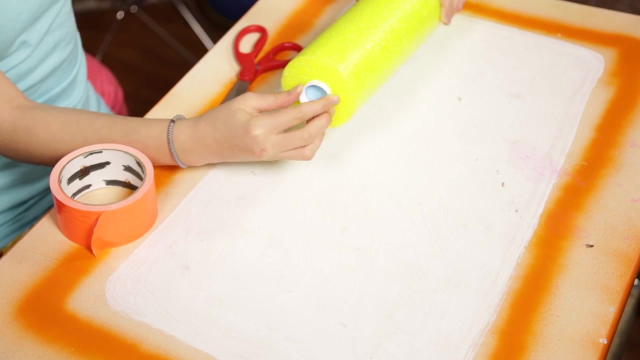 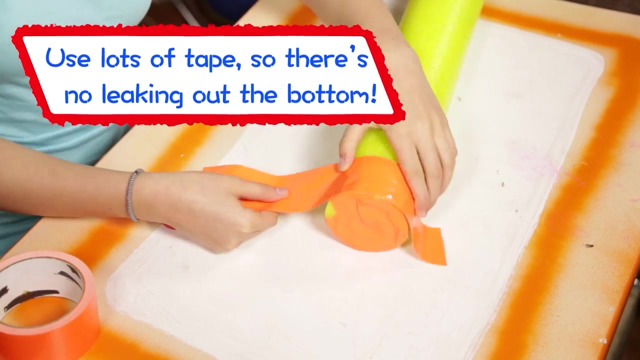 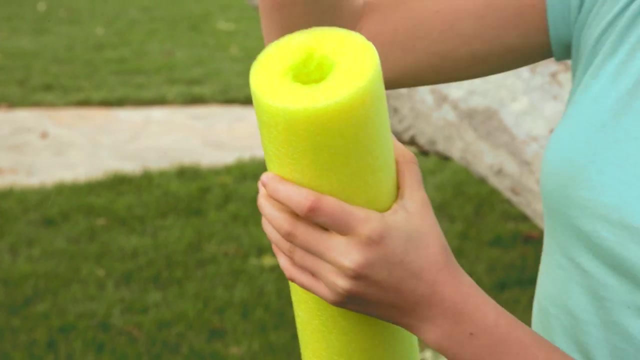 Poke lots of holes into the pool noodle using a chopstick. Next, to make a plug, place a bottle cap into one end of the noodle. Now tape over the plug end of your noodle. Slide the end of the hose into the open end of the noodle. 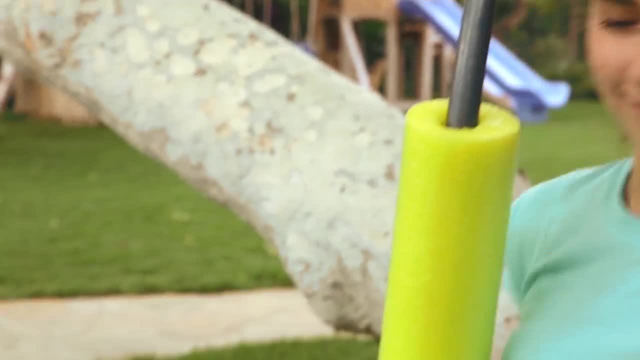 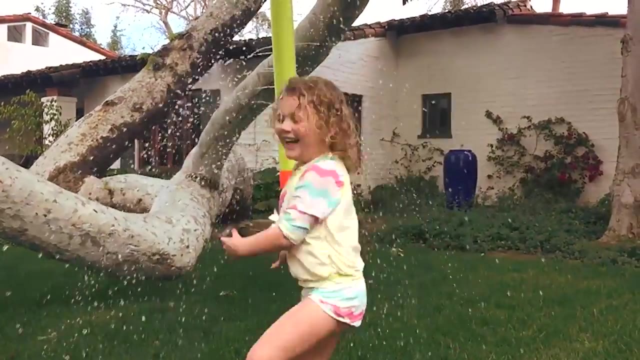 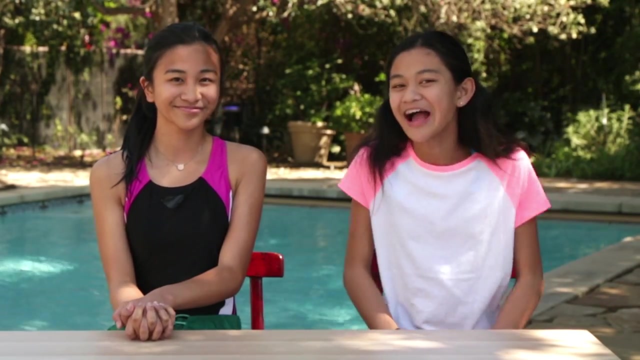 Push it in a few inches so it stays, Turn on the hose and prepare for maximum sunny day fun. I'm Jillian And I'm your sister, Angelina, And today's episode is kicking it back at the pool hacks. Nothing is better than spending the day at the pool. 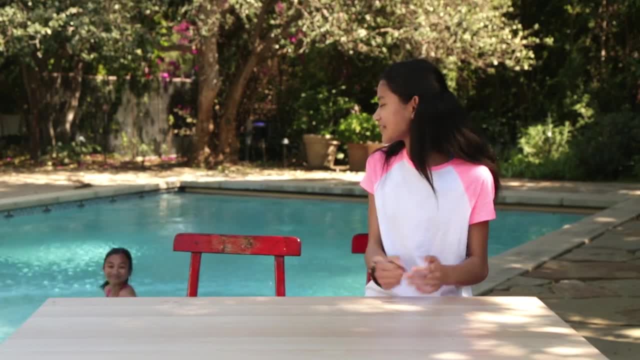 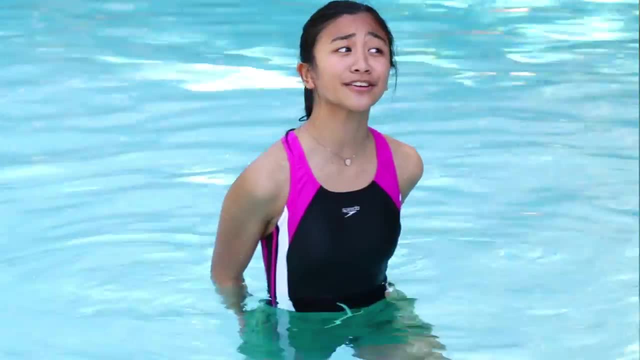 Yes, But Angelina, you were supposed to say that the day can be even better with some great pool hacks. Oops, Well, it seems like you got things under control up there, so I'm just going to sit back here in this cool, refreshing pool. 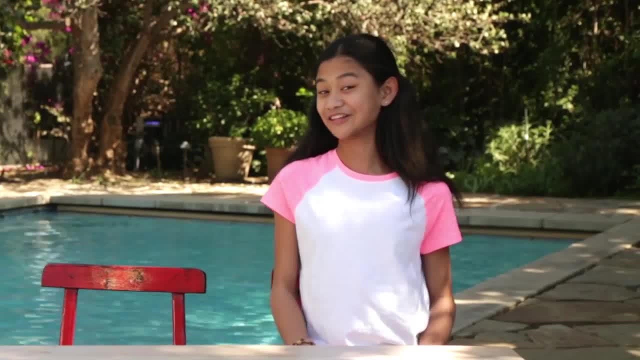 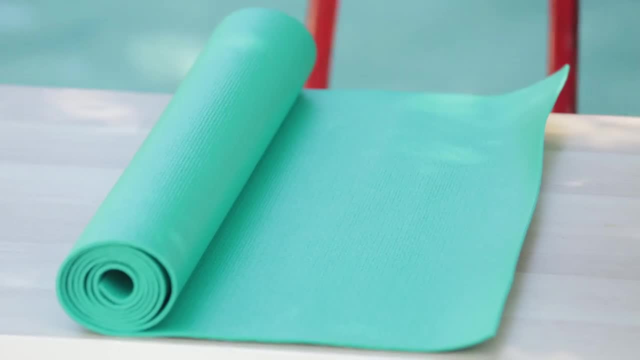 Although it's so bright, I can barely see you. Well, lucky for you, I've got a hack for that that involves an old yoga mat, My Wiser Yoga Mat Visor. For this hack, you'll need an old yoga mat, scissors, a hole puncher and shades. 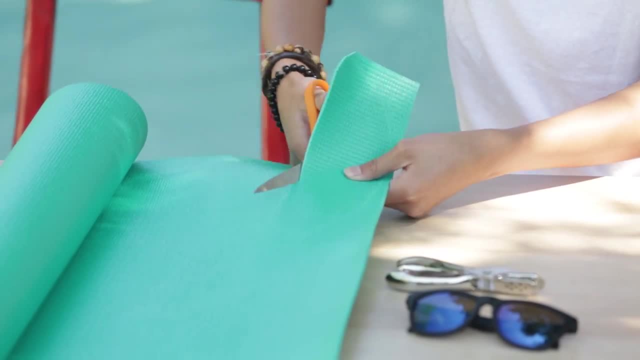 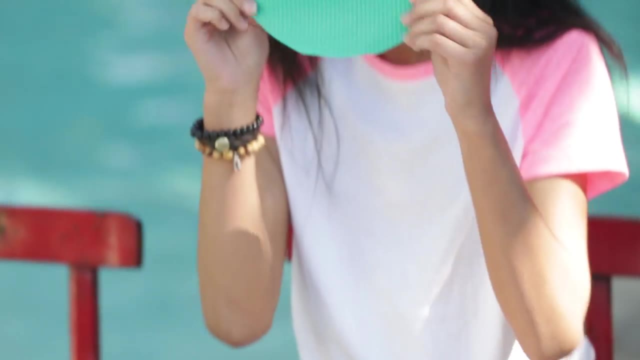 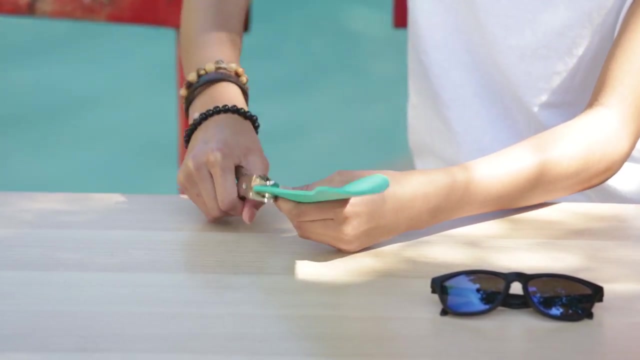 Cut a smile shape. Cut a smile shape out of your yoga mat, about 9 inches long and 4 inches wide. Poke two holes with your hole puncher on either side of your shape. Now open your shades and put it on like this: 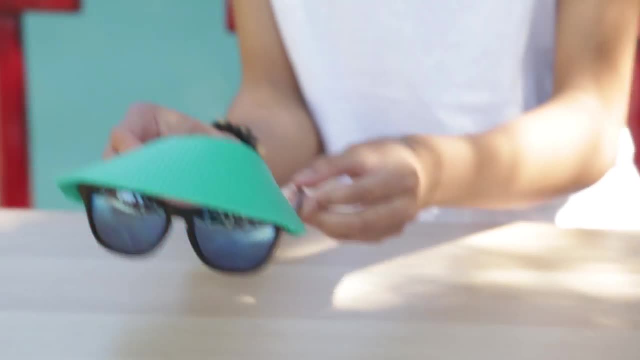 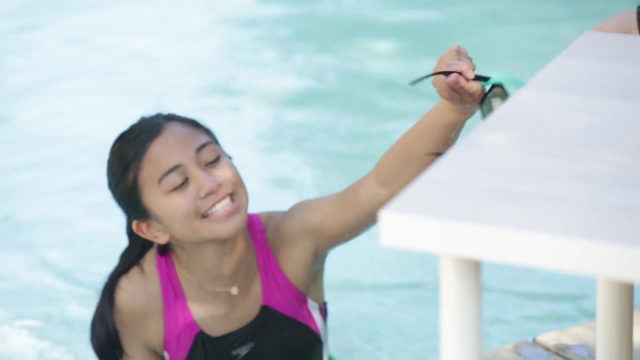 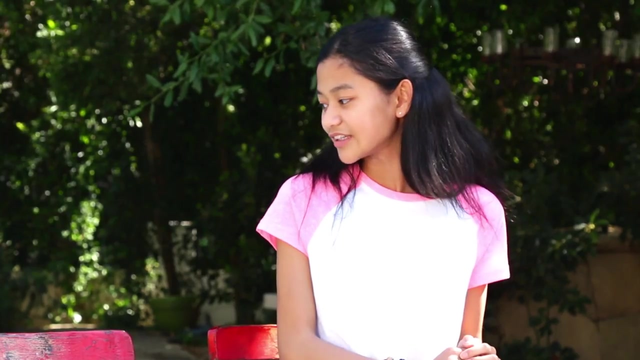 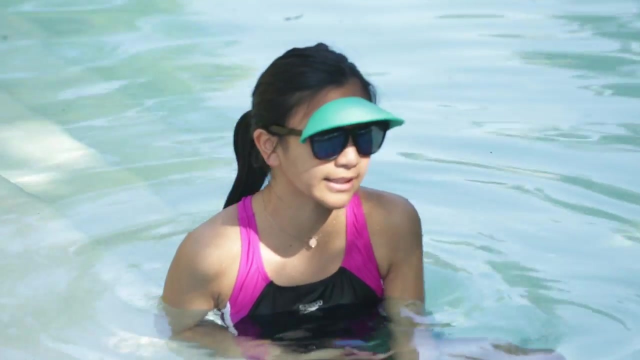 Now you can namaste cool this summer. That's so cool. It's like sunglasses and visor in one. Now for my next hack. I'm Oh Jilly, Yes, Well, now it's not the sun that's bothering me, but I'm really thirsty and it'd be such a bummer to have to get out of the pool and get something to drink. 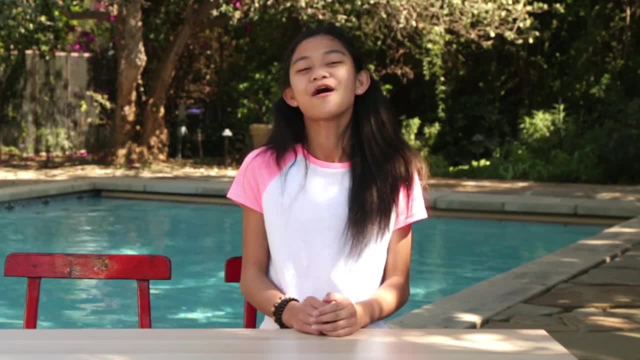 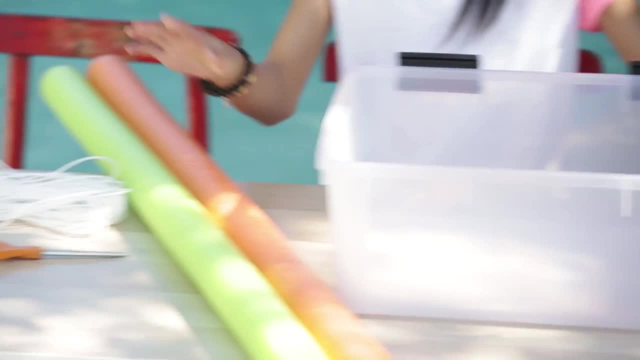 Well, lucky for you, I was going to get something to drink. I was going to make my Cooler Noodle Cooler. For this hack you'll need a plastic storage container that isn't too deep, two pool noodles, waterproof rope and scissors. 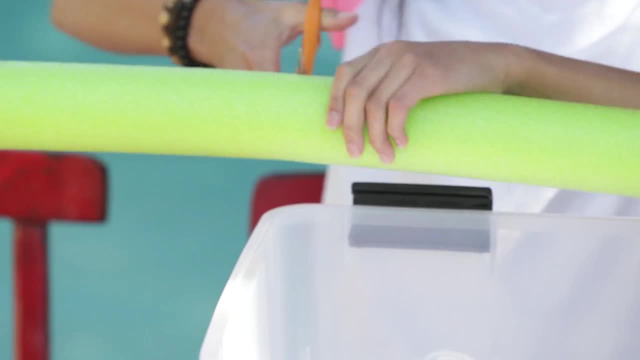 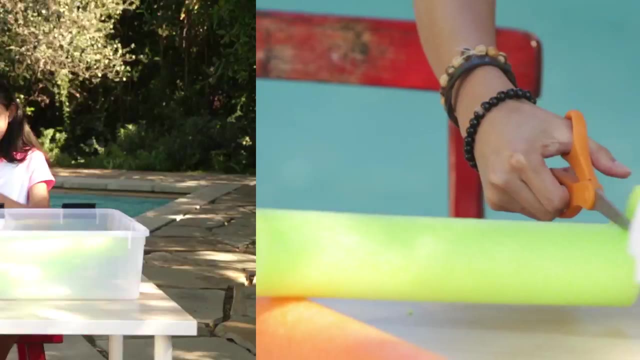 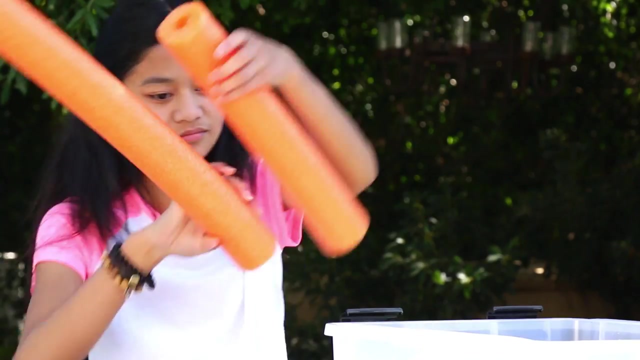 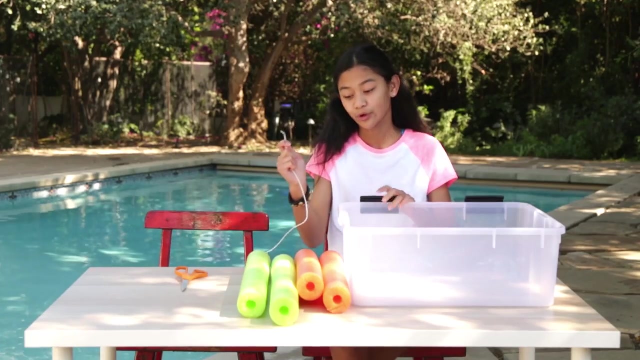 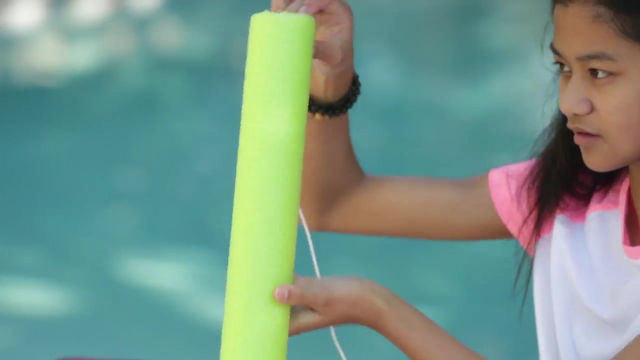 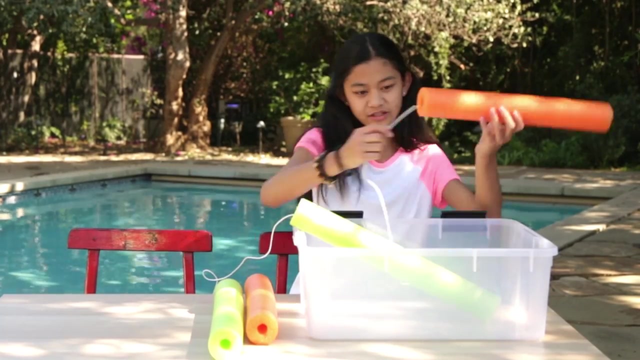 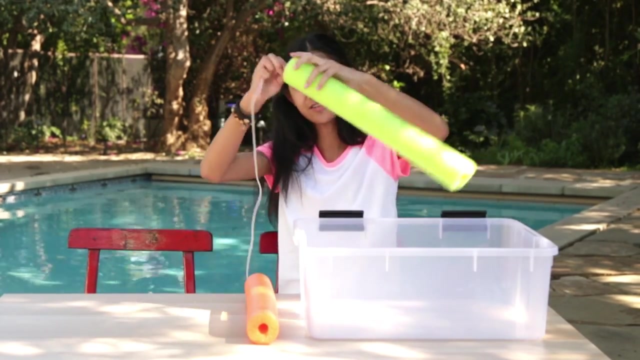 Cut two pool noodles that are equal to the length and two that are equal to the width. Now thread your rope through all four pool noodles, alternating between the length and the width. Now wrap your pool noodles around the lip of the container and tie it in place. 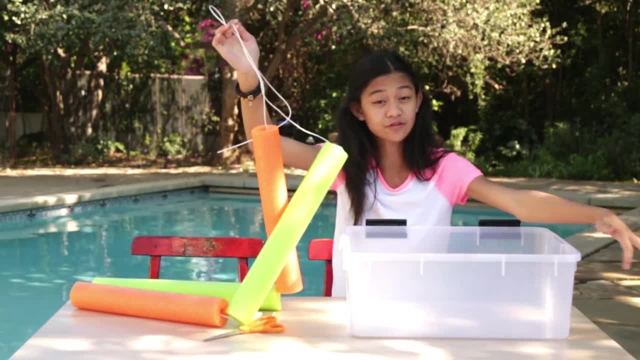 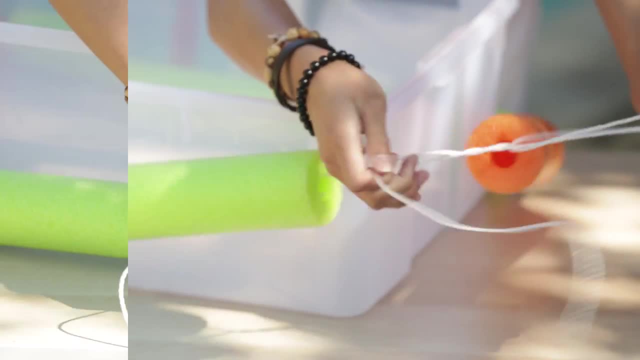 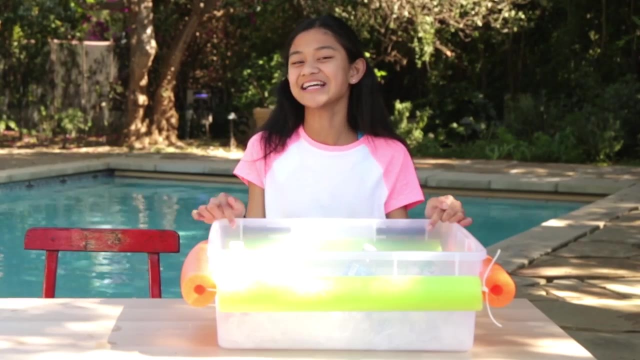 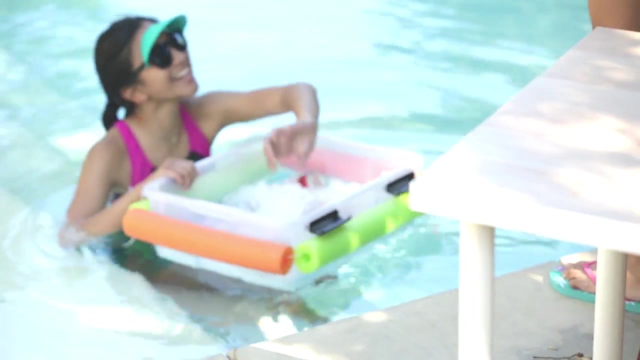 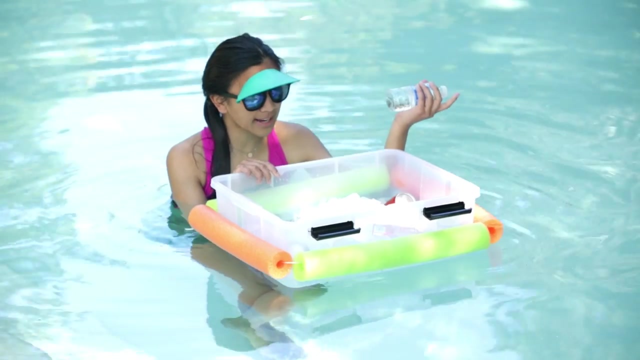 Now wrap your pool noodles around the lip of the container and tie it in place. Now just add ice and your drinks are ready to set sail. Here you go. Thanks again, You're welcome. But Jillian, What now? You call this kicking back at the pool hack, but so far all we've done is work. 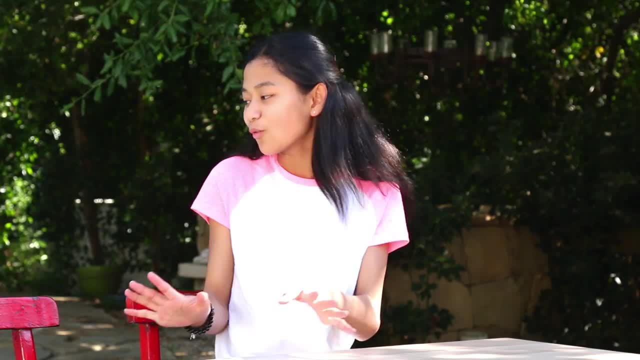 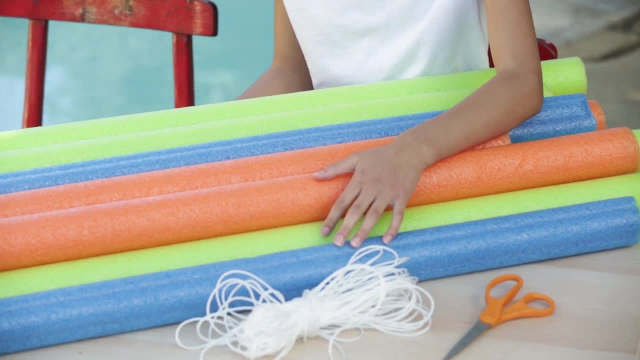 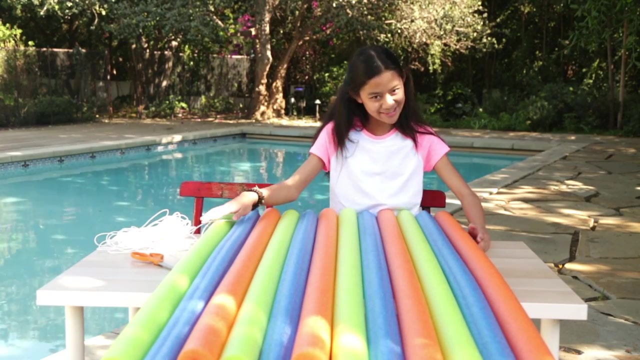 Yes, all we've done is work. Well, don't worry, because you'll be relaxing on your back in no time, flat with my relaxing raft. For this hack you'll need 12 pool noodles, waterproof rope and scissors. Lay out your 12 pool noodles like this: 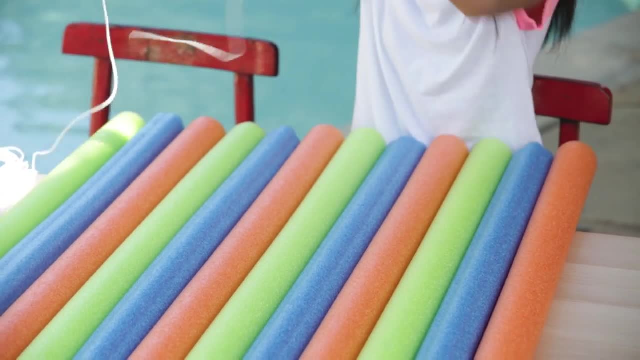 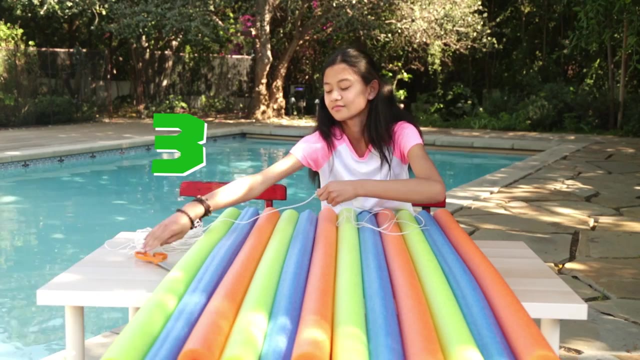 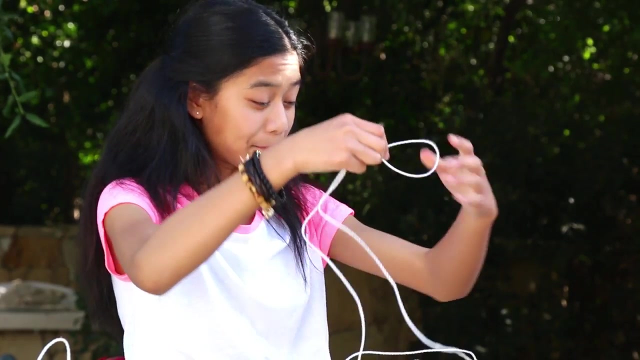 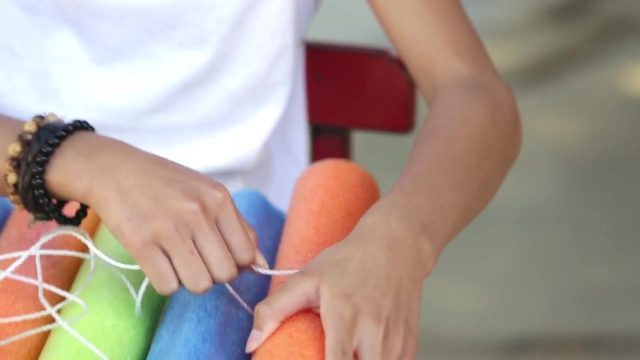 Now take your string and measure about three times the width. Okay, Lift your rope in half and then, where you folded it, wrap it around the end of your pool noodle And make sure to push it about six inches like this, And then tie one knot. 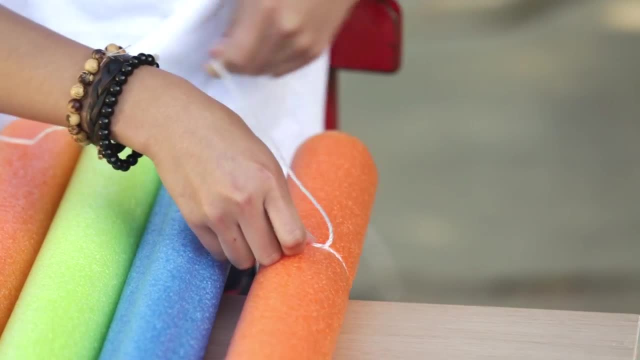 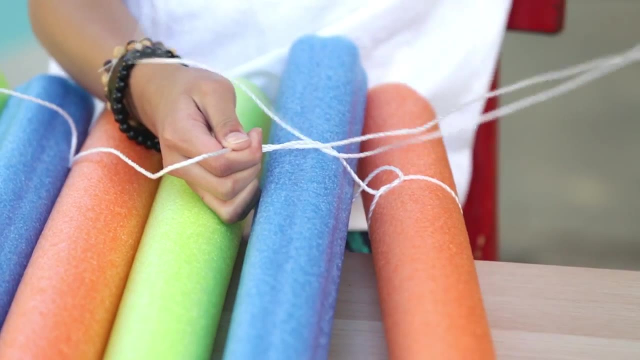 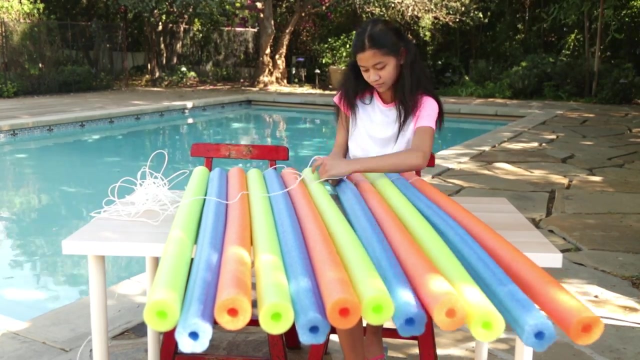 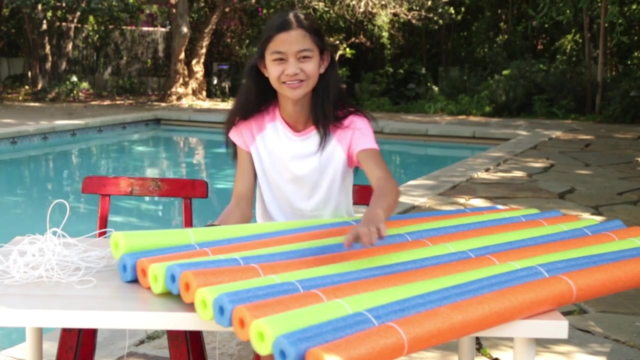 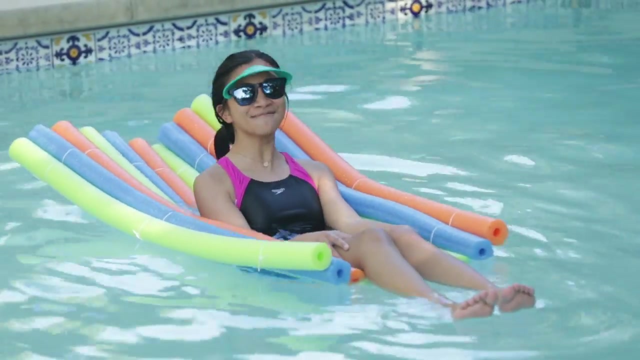 Pull it kind of tight and then repeat this step for the rest of your pool noodles And then trim off the end. Repeat this in the middle and at the other end, My relaxing raft. Let's kick off. this kicking back Looks like I'm going to make another raft for myself. 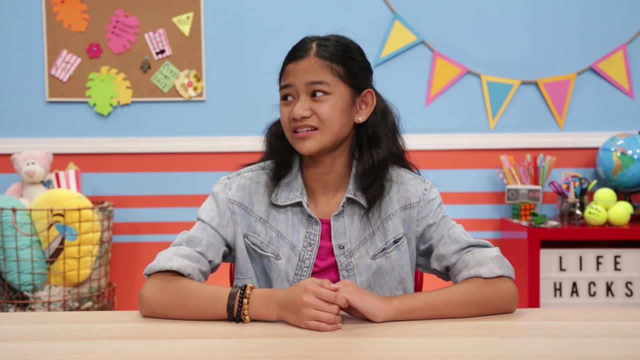 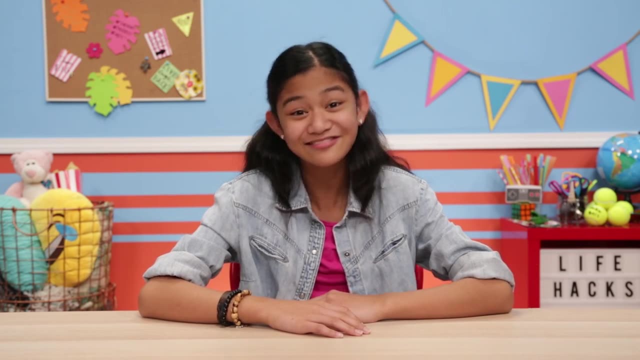 Living in the city can be noisy, Noisy, But I like parks, fresh air, open space, green grass- what's not to love? So today we'll make some hacks for your next park day, in the sun and on the grass. 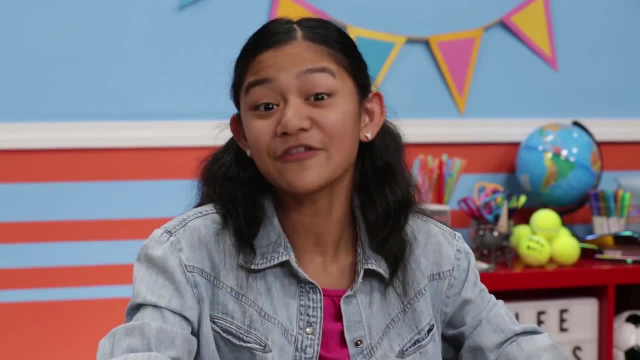 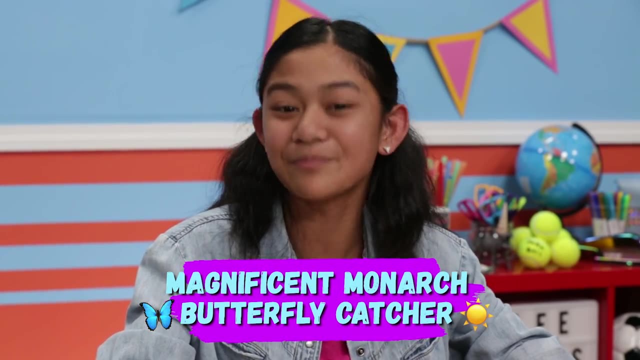 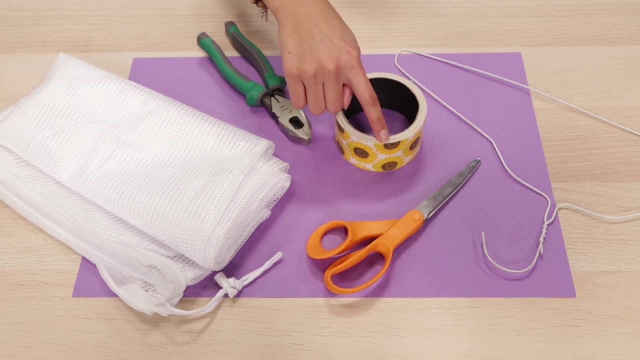 These are my. park it and have fun hacks. My first hack is so good, it gives me butterflies. literally, It's my magnificent monarch butterfly catcher. For this you'll need a mesh laundry bag, pliers, duct tape- I'm using a fun pattern- scissors. 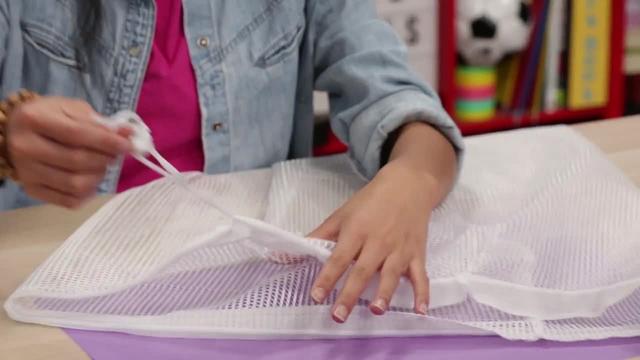 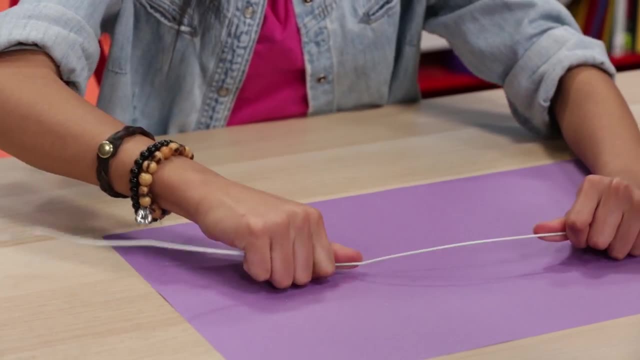 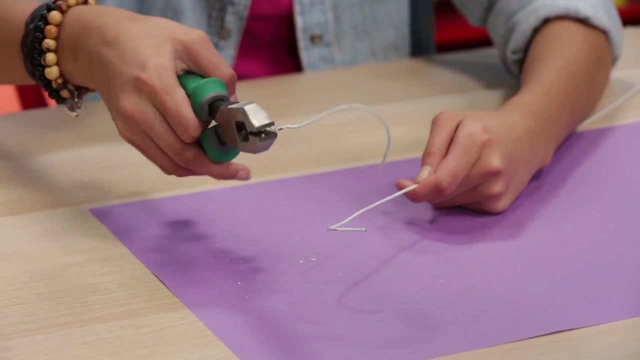 And then a wire coat hanger. Cut the string out of your mesh laundry bag, Set it aside. Straighten out a hanger. Snip the curly ends off. Bend one end into a little loop. This will make it easier to feed through your mesh bag. 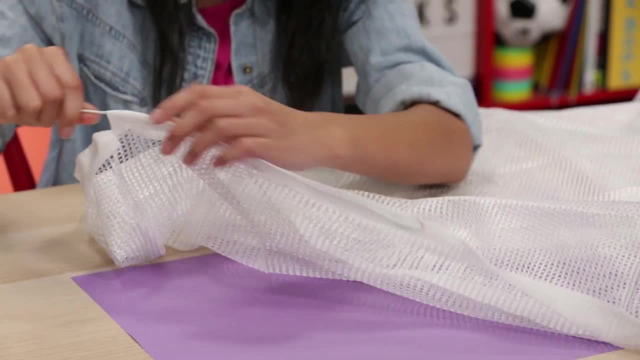 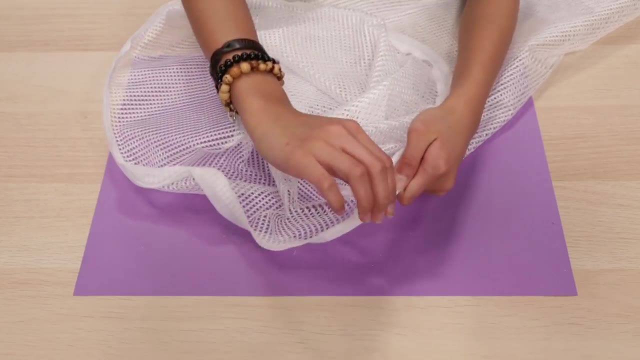 Thread your loop side through the laundry bag where your string was. Bend the hanger into a string. Bend the hanger into a string. Bend the hanger into a string. avez Loop it around. Bend the bottom end so it doesn't slip through the mesh. 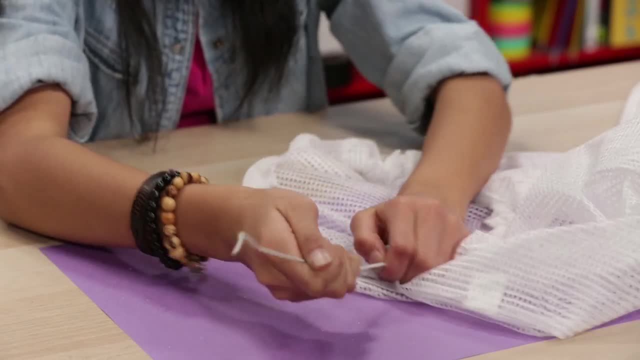 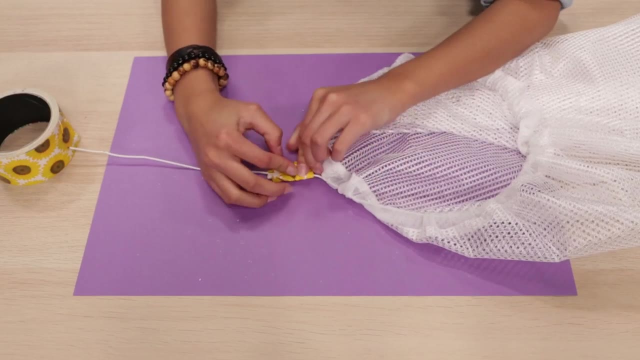 Thread the straight end of the wire through the loop and then pull it to make the circle smaller. once you get the size that you want, tape it in place. Then tape up the rest of your handle. If you have a really big laundry bag, like I do, just tie it where you want it to stay. 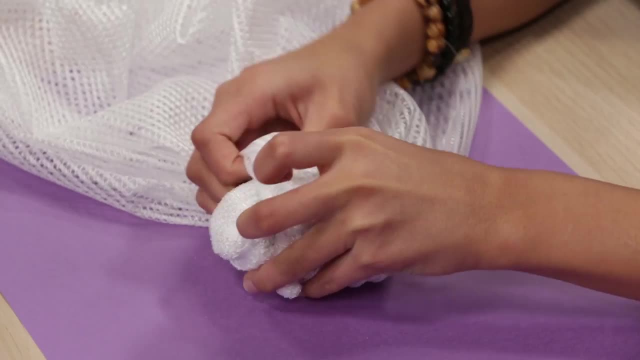 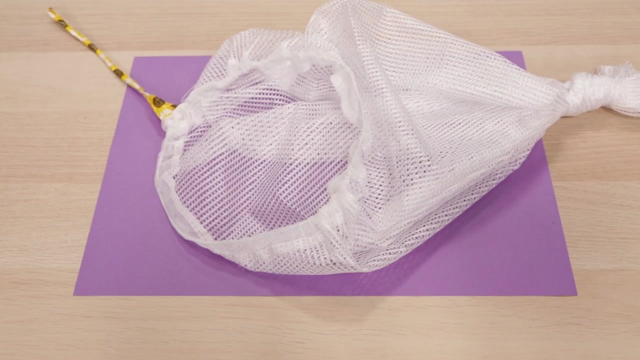 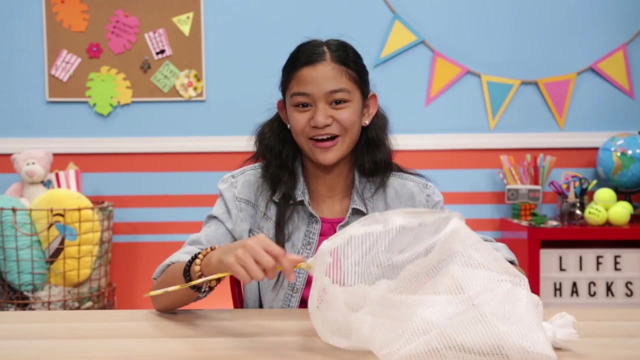 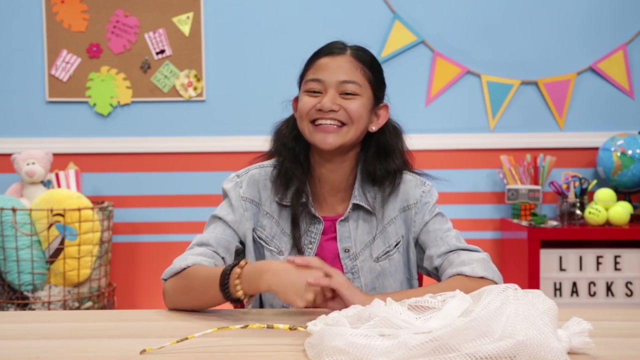 big laundry bag like I do. just tie a knot and then cut the excess off. Oh hey, what did the butterfly say to the flower? Hey, bud. Up next is a hack that will make it easy to hang in the sun all day. 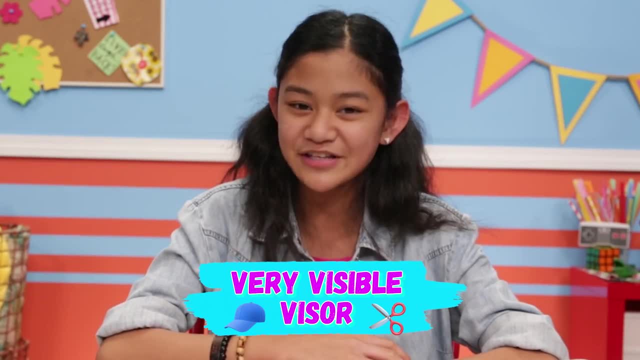 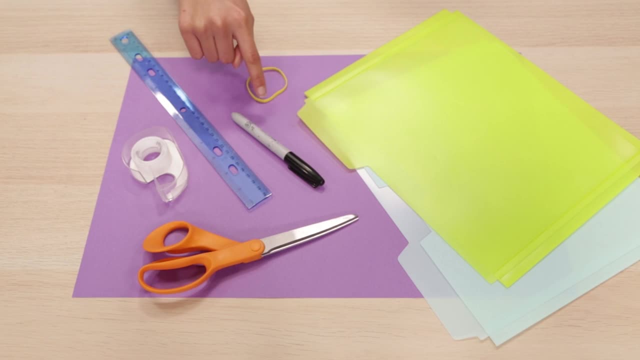 while keeping those pesky rays away. It's my Very Visible Visor. For this you'll need scotch tape, a ruler, a pair of scissors, a rubber band, a marker and two plastic folders. First, make your strap. 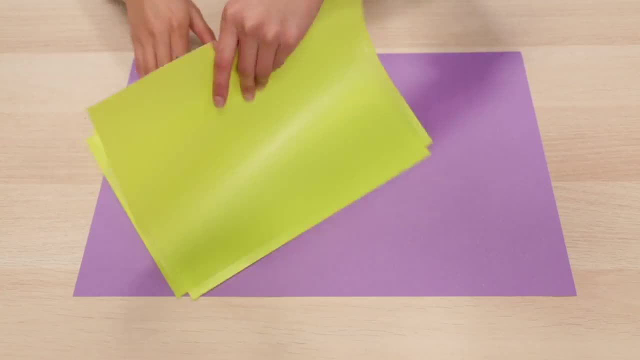 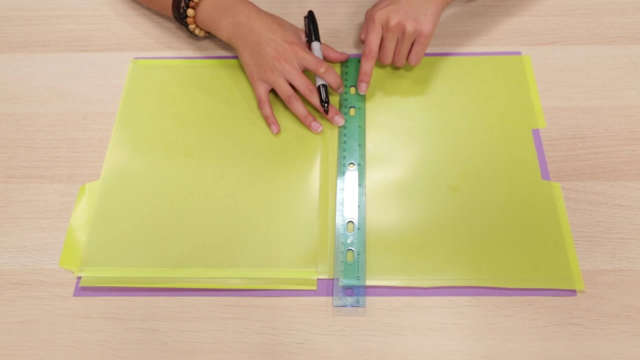 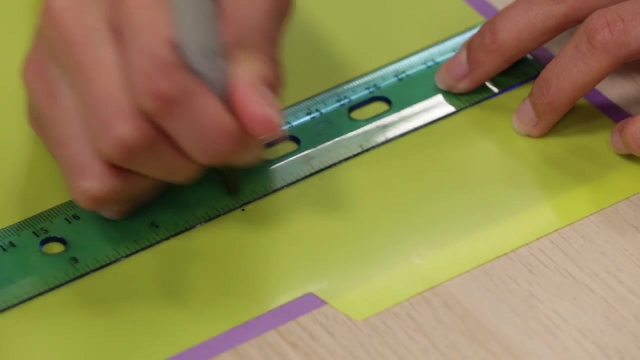 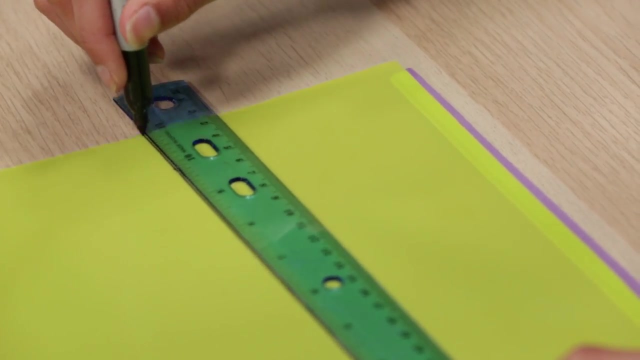 Cut the closed edges of your folder so it can lay flat. Cut one side so it's completely straight. Use a ruler to measure a four-inch strip, Not a wing, just a fifth. Now we're going to cut noodles. The best way to do this is to cut through the 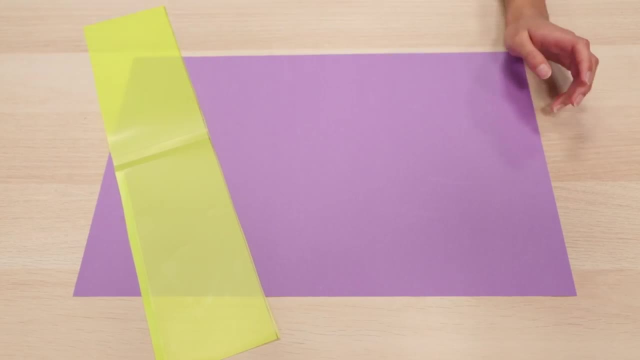 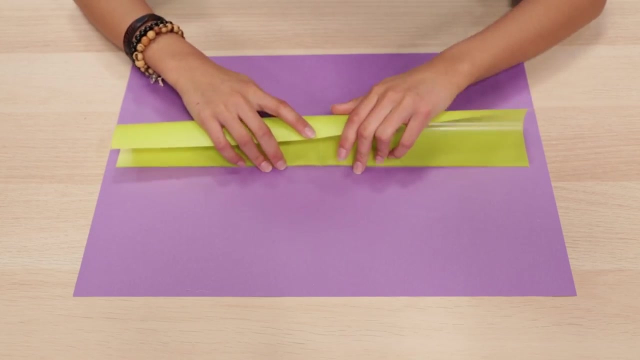 Cut it out. Trim the edges so they're even. Fold the strip in half, hot dog style. Set it aside. Trim the edges, so they're even. Trim the edges so they're even Hold the strip in half- hot dog style. 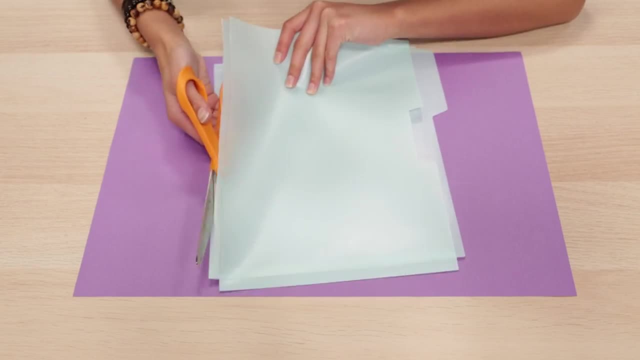 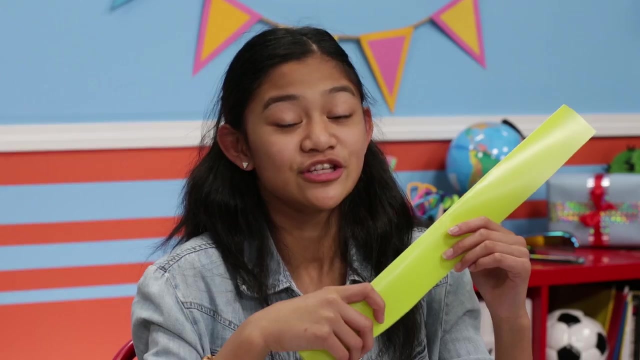 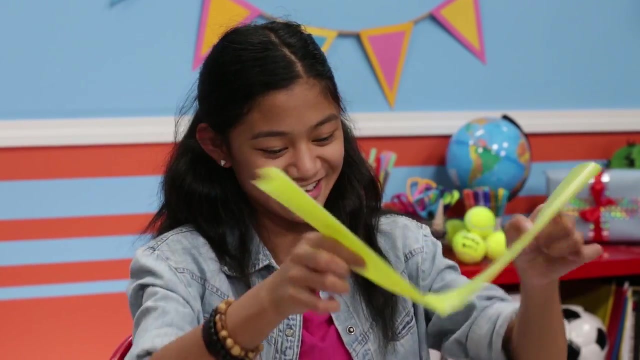 Hold the strip in half, hot dog style, and set it aside. bill Trim off one side of your folder. Cut all the edges so they're straight. Use your visor strap to measure how big your bill should be. Make two marks where you. 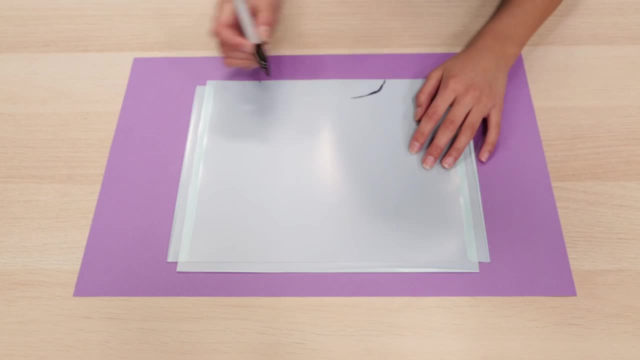 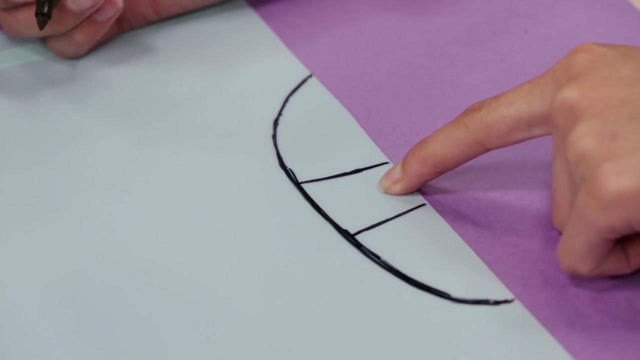 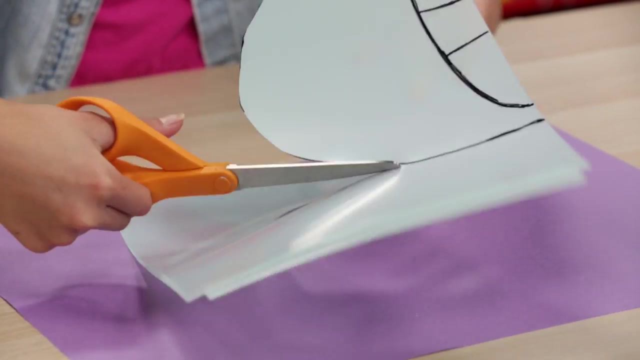 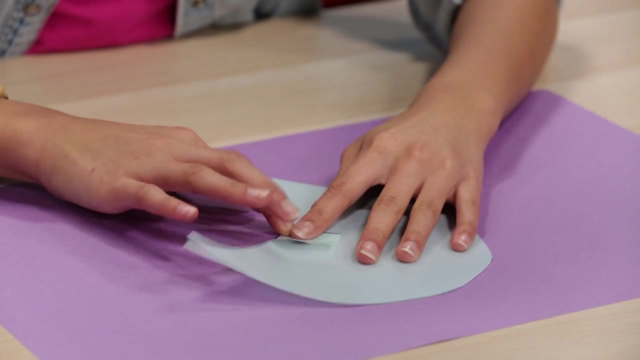 measure and draw a curved line between the two marks. Add a tooth in the middle of your arch. Draw your bill whatever shape you want. Cut it out and don't cut the tooth. Bend the tooth over so it's sticking straight up. 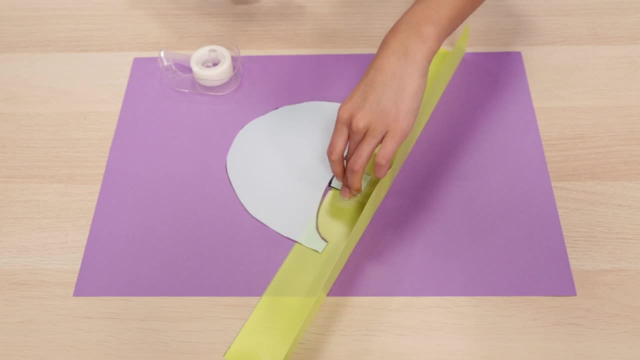 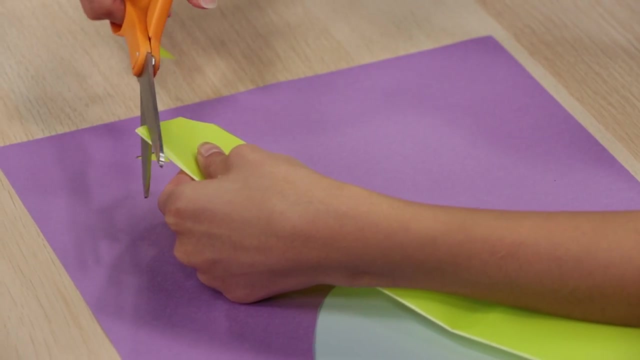 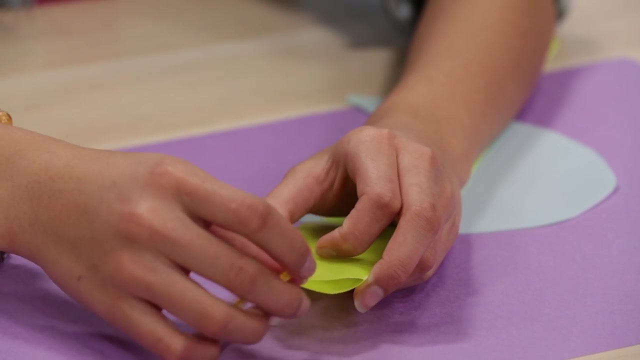 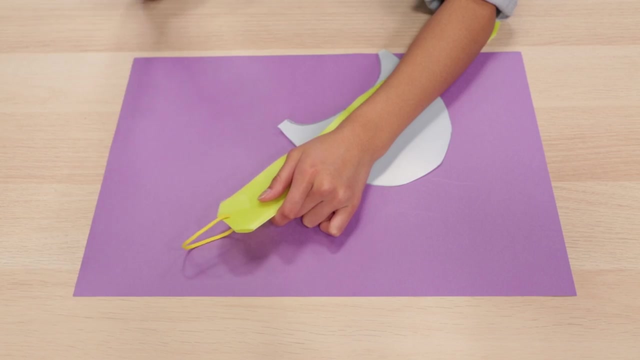 Stick the tooth inside the strap and tape it down. Fold the strap over. Trim off the corners. This will make it more comfortable to wear. Cut a slit in the edge of your strap and slip your rubber band through. Then tape it closed. Do that to the other side and feed. 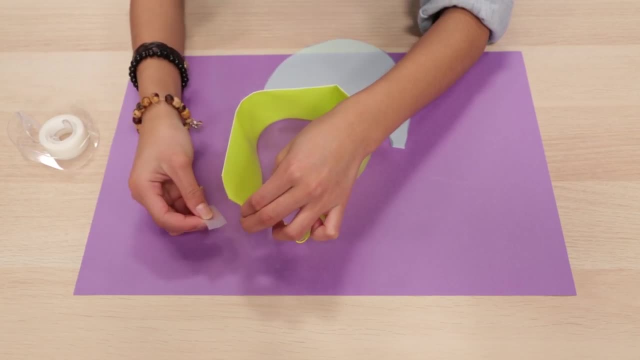 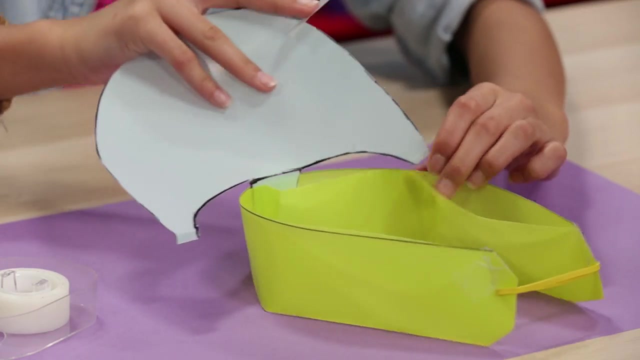 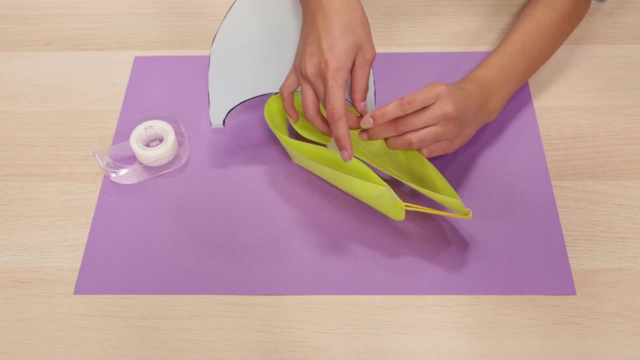 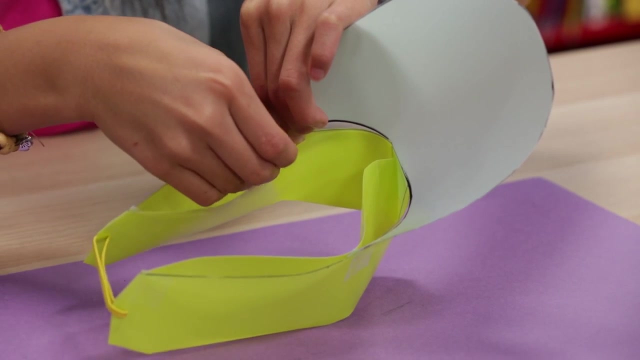 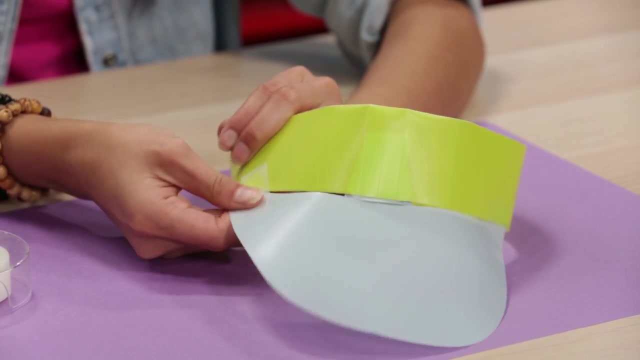 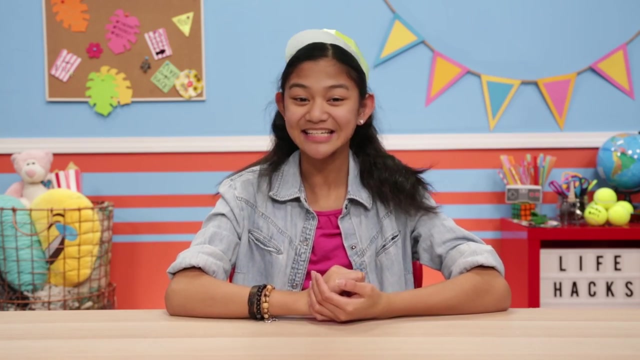 your rubber band through so they connect. Tape that closed too. Tape the ends of your bill to your strap. Try to tape it in between the layers. This visor's got me brimming with excitement for what's next. To add a bit of activity. 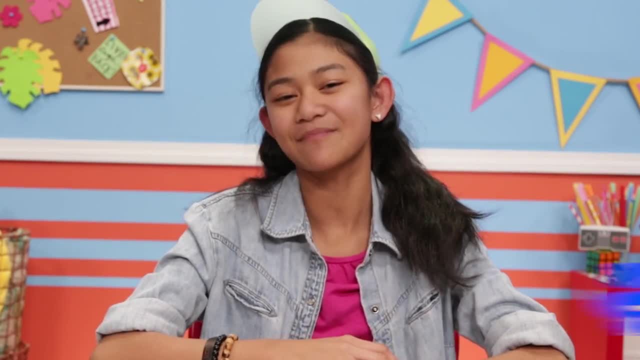 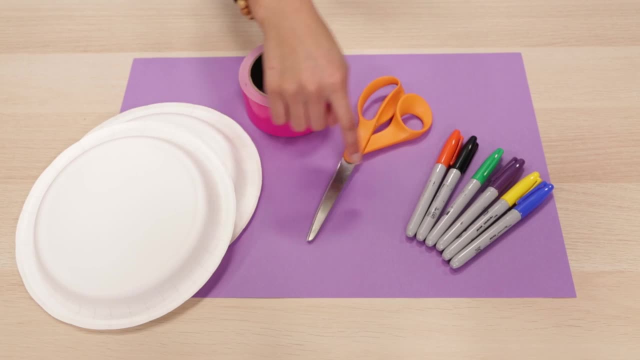 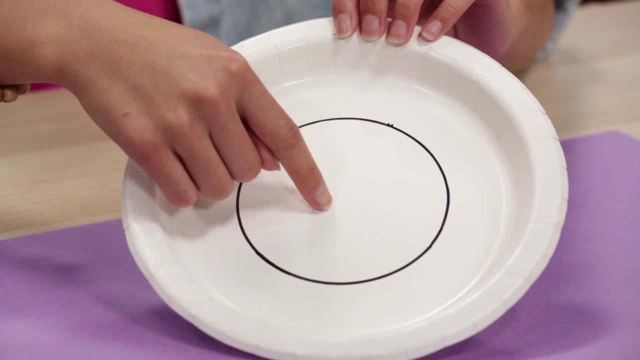 to your day besides just a walk in the park. let's hack my easy peasy frisbee. For this you'll need two paper plates, duct tape, scissors and colored markers. Use a roll of duct tape to trace a circle in the middle of your plate. Cut it out. 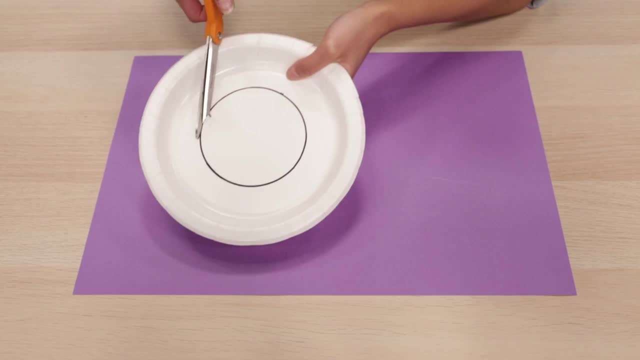 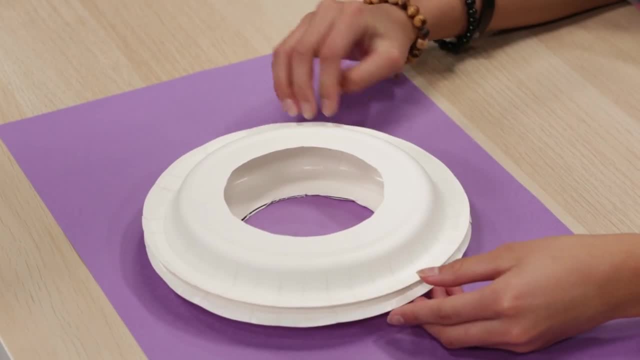 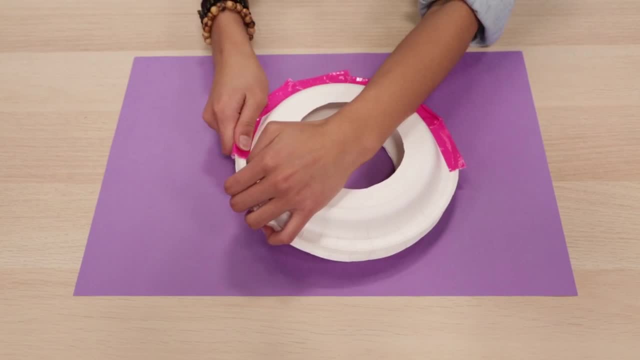 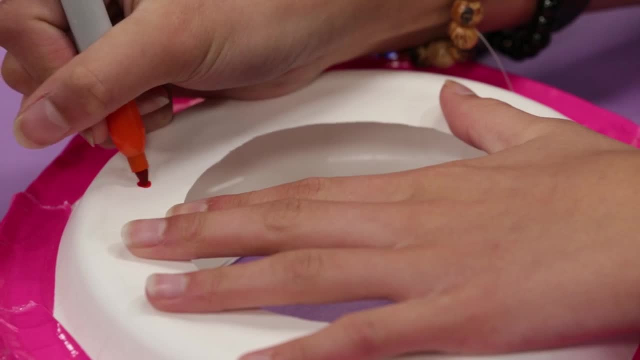 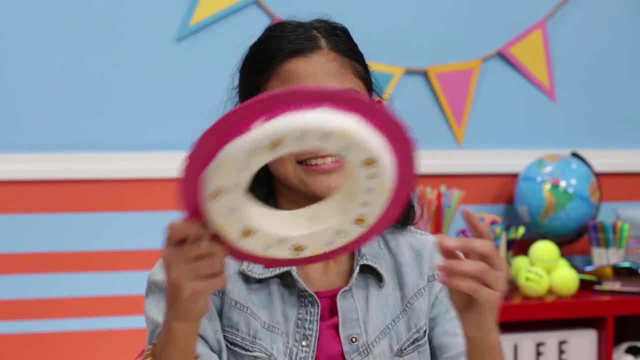 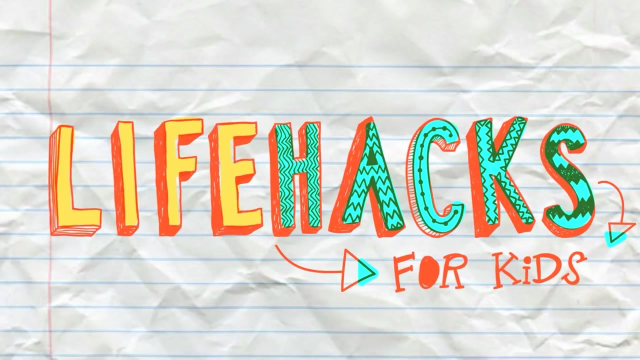 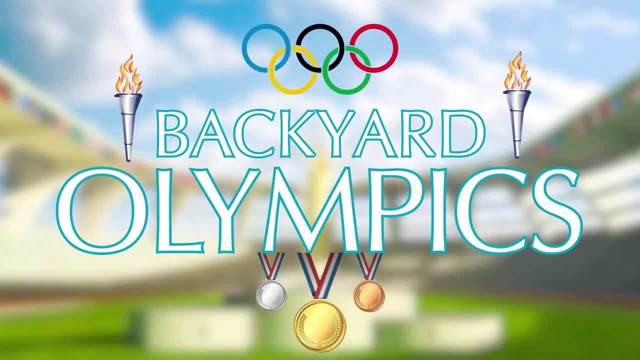 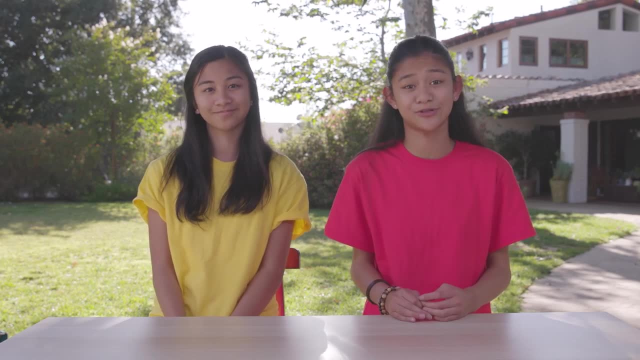 And today's episode is Backyard. Only Wait, I want the gold. Well then, you're going to have to earn it, because I need help making some backyard obstacle courses. I'm in First up human ring toss Angelene, how are your lungs? 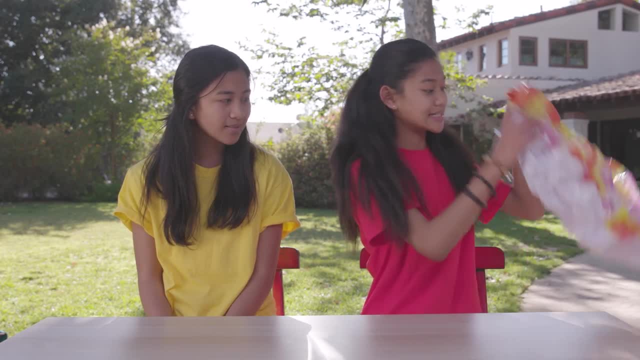 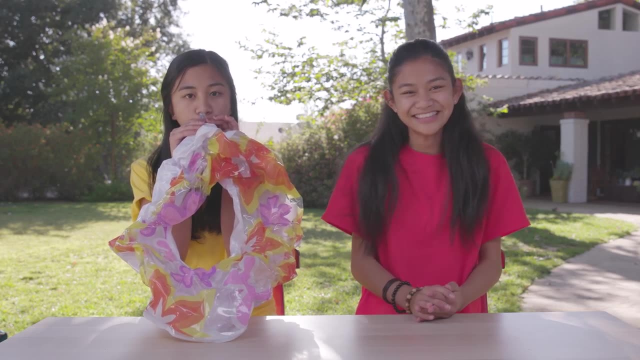 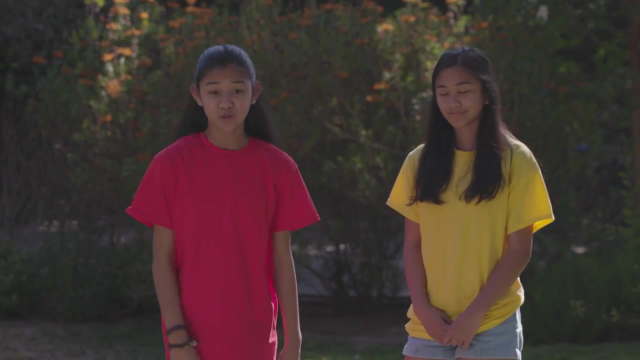 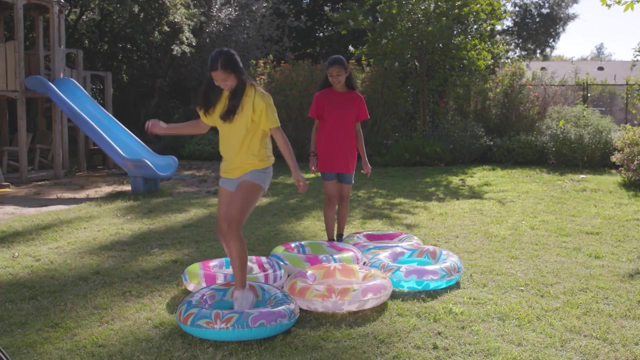 Why do you ask? Well, we're going to need six of these blown up. Set your tubes in a row like this: In the course, run across the tubes, making sure that your feet are in the middle of the holes When both you and your partner get to the end. 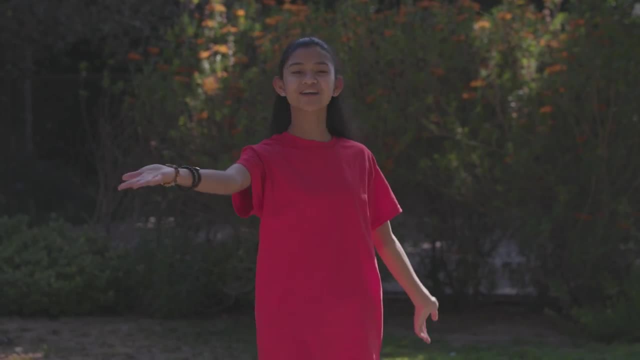 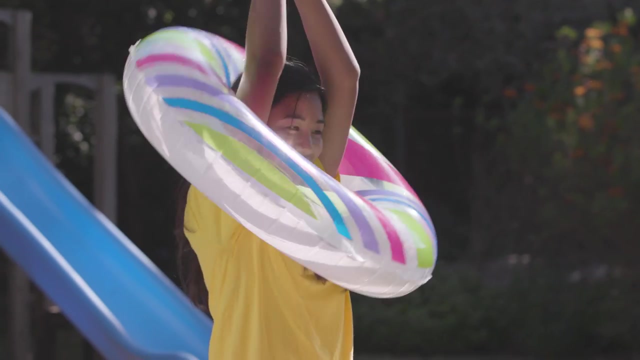 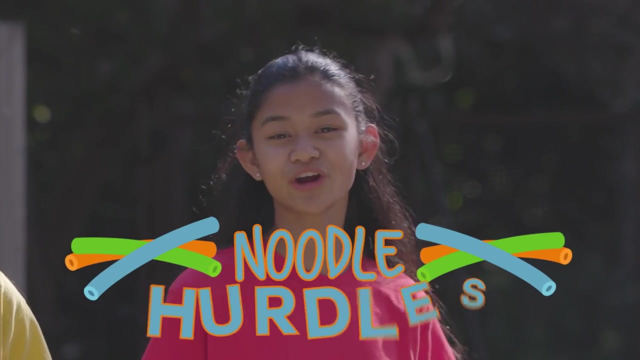 play human ring toss and make sure you get at least three on your partner: One, two, three. The next part of the course is noodle hurdles. To make your noodle hurdle you'll need two baskets or buckets that are the same size. 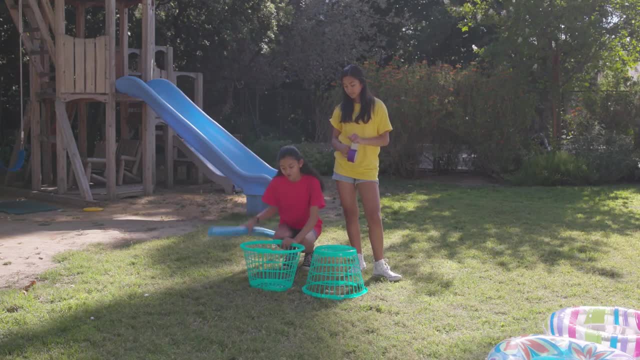 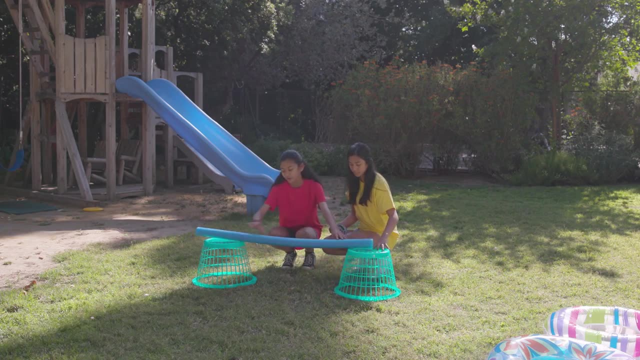 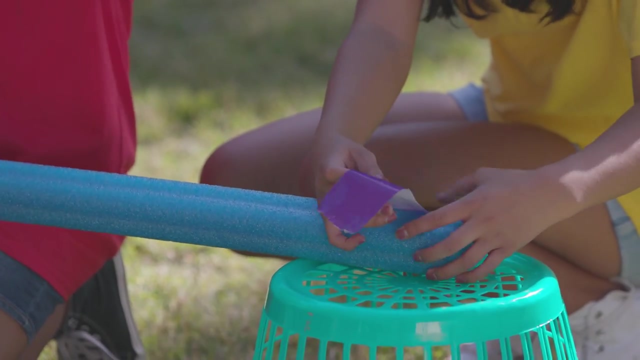 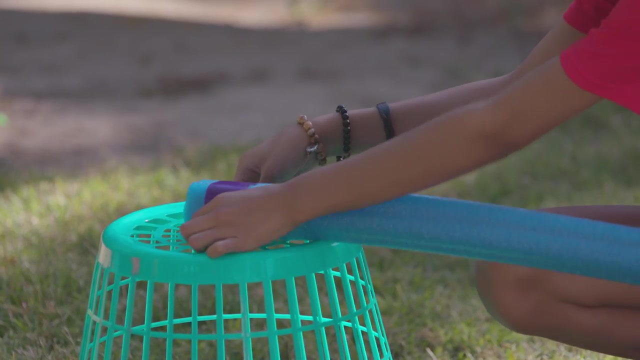 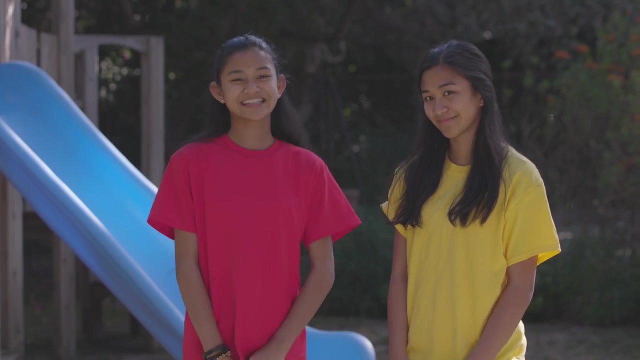 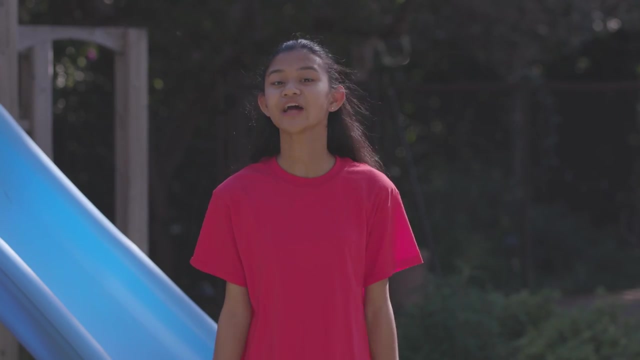 one pool noodle and duct tape. You turn over both your basket or bucket And keep them at an equal distance, And then you tape the pool noodle on top And you're done. Try it with different sizes of buckets. To go through this obstacle, all you have to do is jump over each pool noodle. 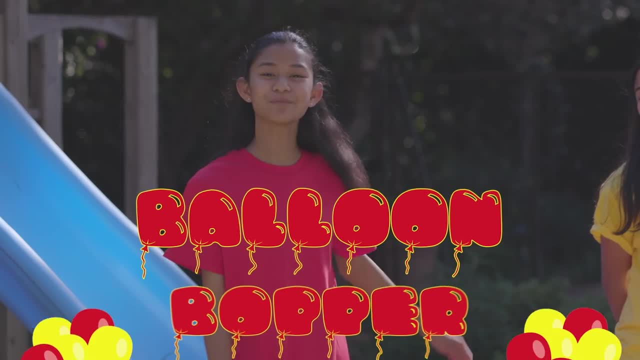 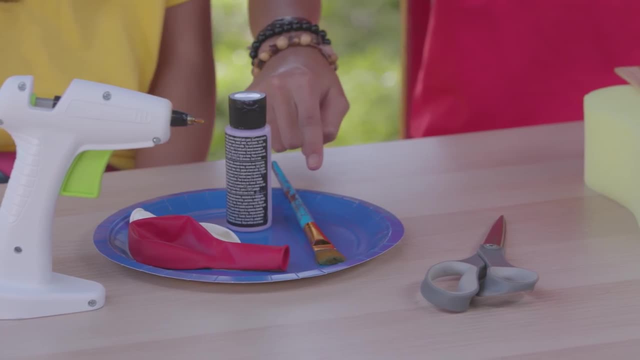 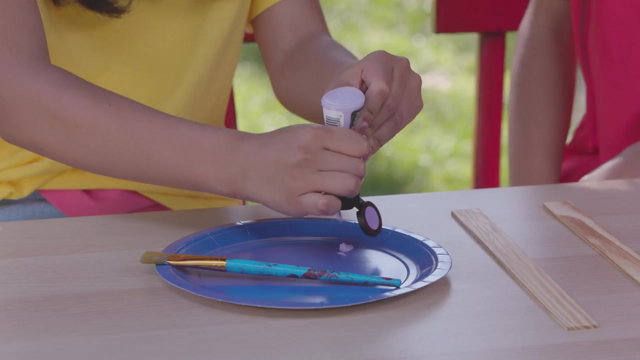 Let's build our final team challenge: the balloon bopper. For this hack you'll need a hot glue gun, balloons, paint, a paintbrush scissors, two paint stir sticks and two large sponges. First, paint your stir sticks. 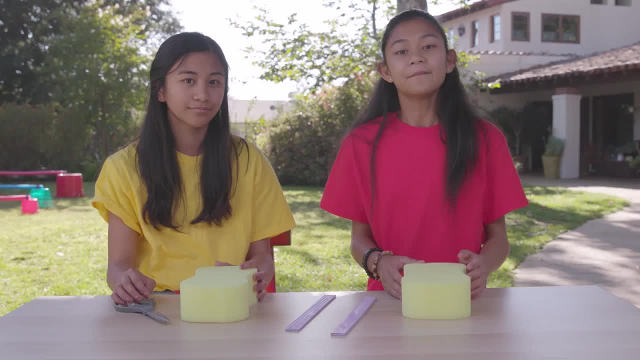 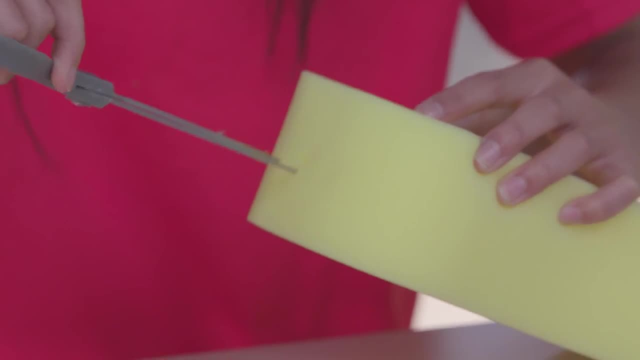 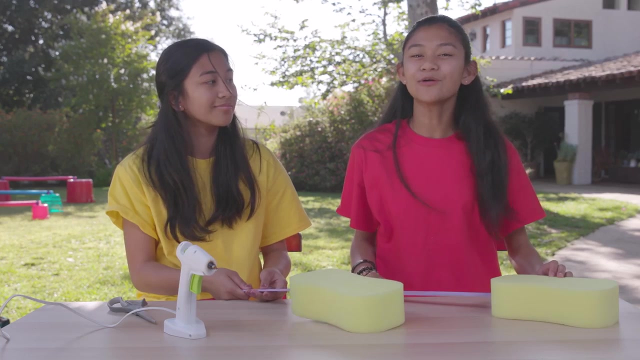 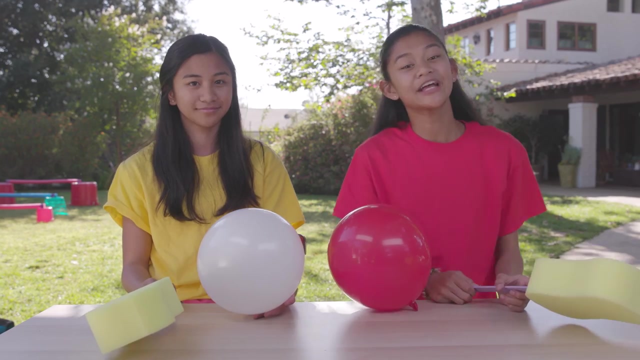 And let them dry. Make a slit in one end of the sponge with your scissors. Now squeeze some hot glue on the end of your stick and then stick it inside your sponge. While that's drying, blow up a balloon To play. hit the balloons back and forth with your boppers. 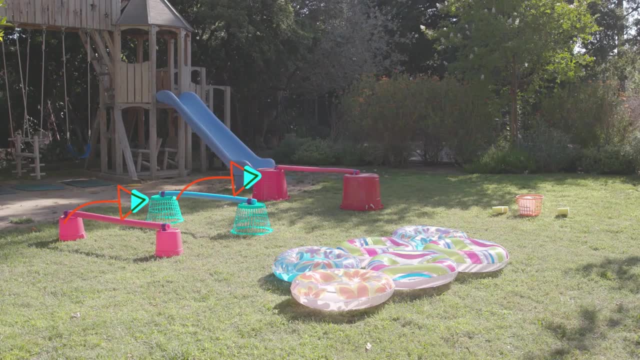 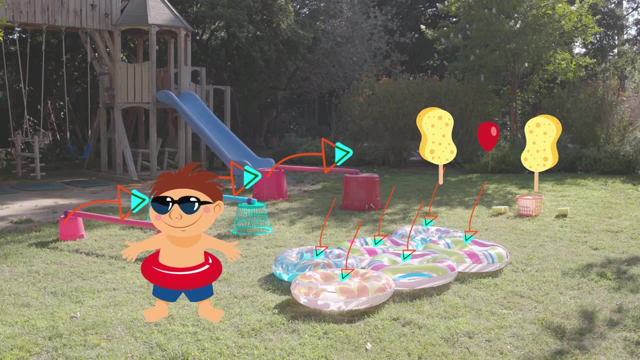 Here's how the course works. First you go through all the balloons, Then you hit the balloon, Then you hit all three turtles, Then you play with the balloon and you bop it four times. You go through the tube and then you play human ring toss with both you and your partner. 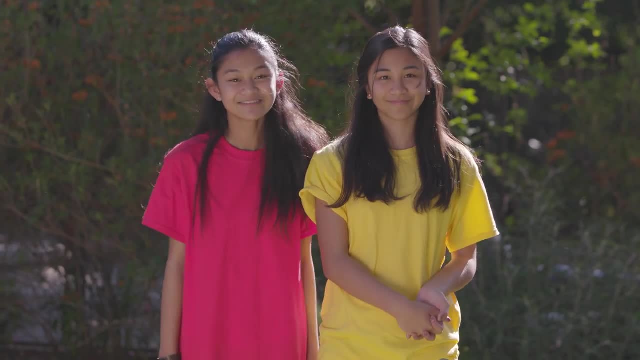 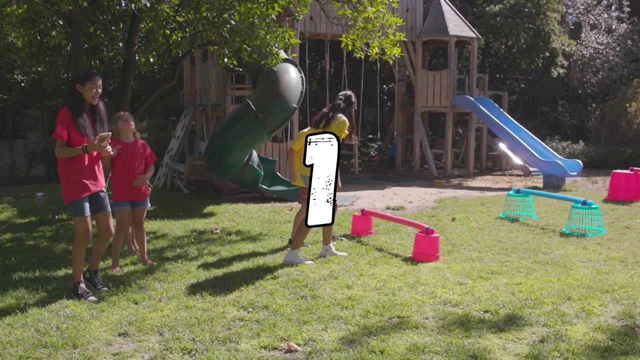 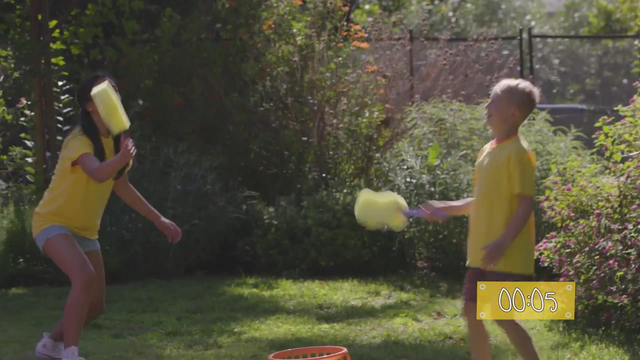 Make sure you get three tubes on your partner, Then you're done, Ready, set. go Four times guys: One, two, three, four go. Shorter person is the ring-toss. Shorter person is the ring-toss. 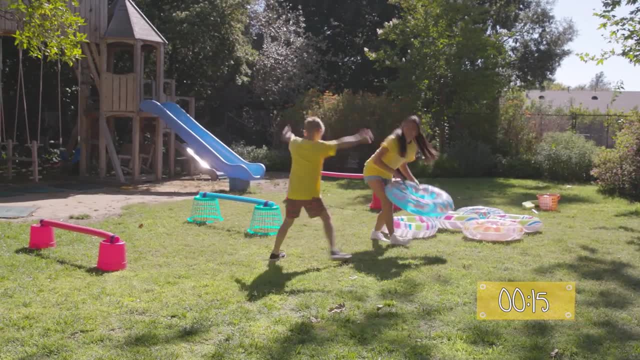 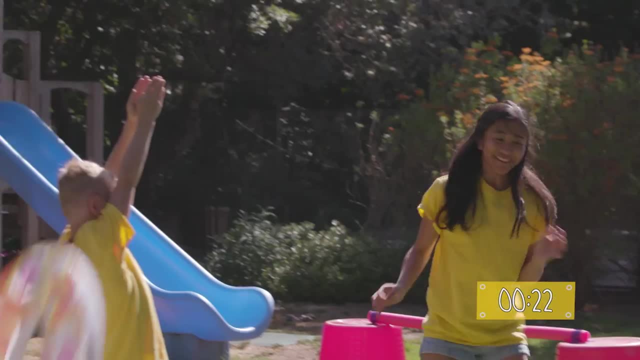 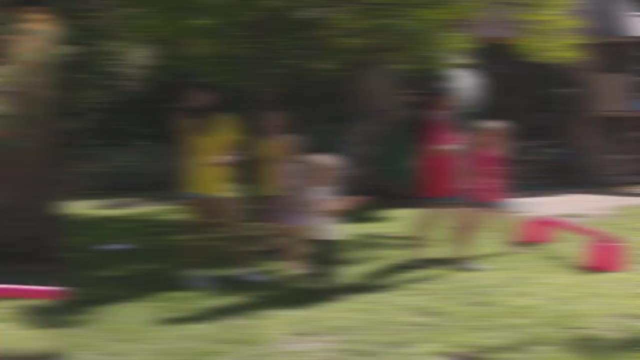 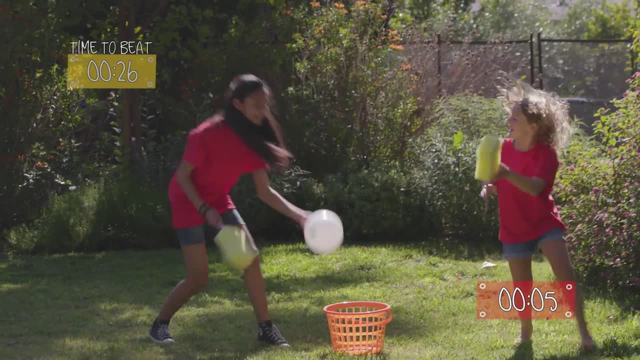 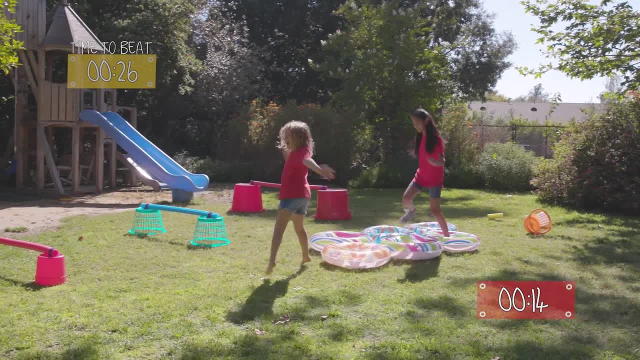 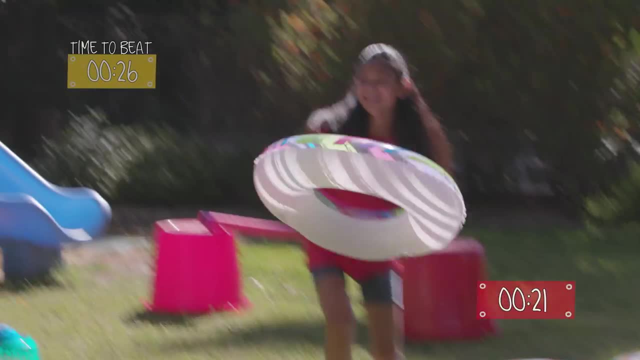 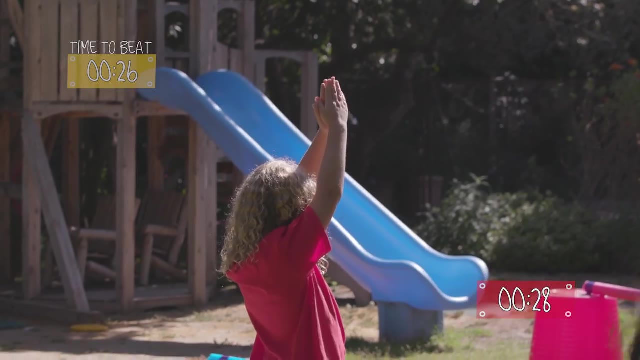 Oh gosh, One, Two, Three, Four, Five, Six, Seven, Eight, Nine, Ten, 11., 12., 13., 14., 15., 16., 17., 18. 19.. 20., 21., 22., 23., 24., 25., 26., 27., 28., 29., 30., 31., 32., 33., 34., 35., 36.. 37., 38., 39., 40., 41., 42., 43., 44., 45., 46., 47., 48., 49., 50., 51., 52., 53.. 54., 55., 56., 57., 58., 59., 60., 61., 62., 63., 64., 65., 66., 67., 68., 67., 68.. 69., 69., 70., 71., 72., 72., 73., 73., 74., 74., 75., 76., 77., 78., 79., 80., 81.. 82., 83., 84., 85., 86., 87., 88., 89., 90., 91., 92., 92., 93., 93., 94., 94., 95.. 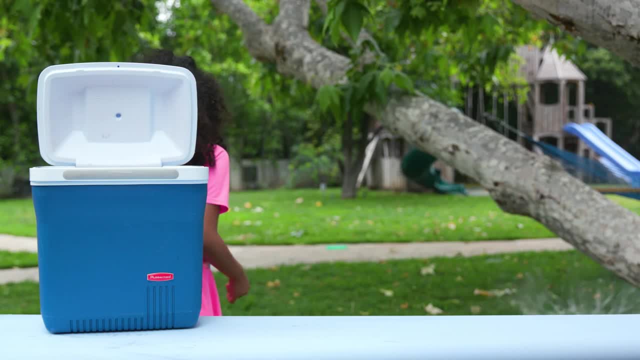 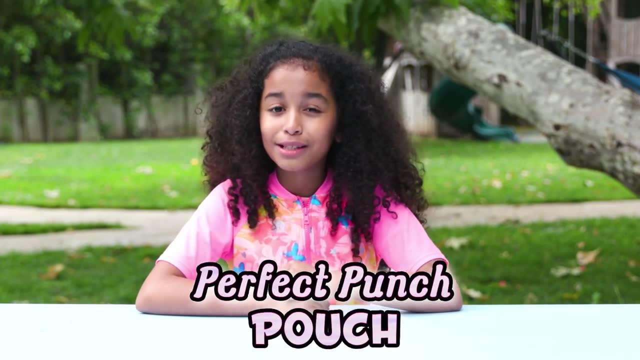 96., 97., 98., 99., 100., 100., 100., 100., 100., 96., 100., 100., 101.. On the couch, It's my Perfect Punch Pouch.